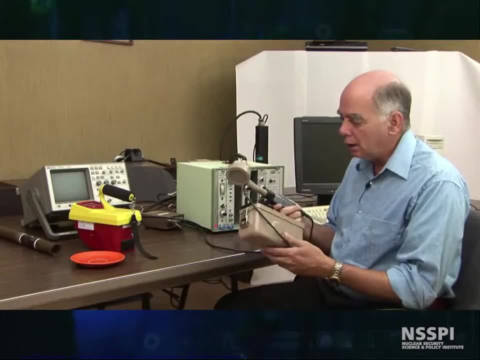 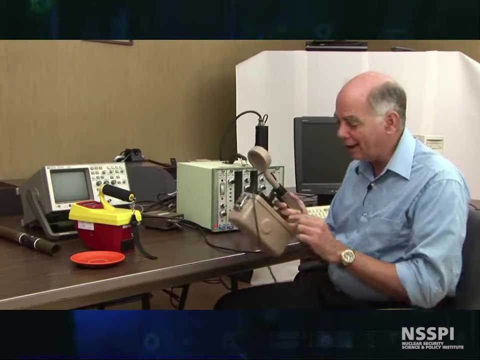 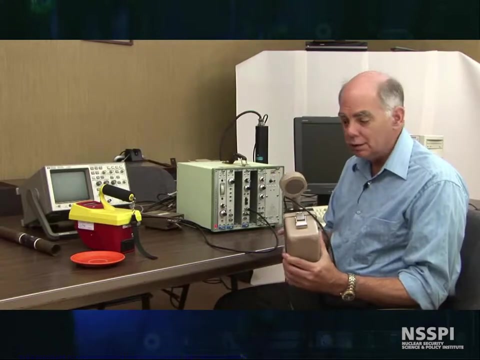 play with is the Geiger counter. here You can have them all hooked up with NIM bins, like you see here, but this one is your basic handheld Geiger counter, and it seems that there's radiation in the room. Well gosh, Since we're here to study uranium, I have 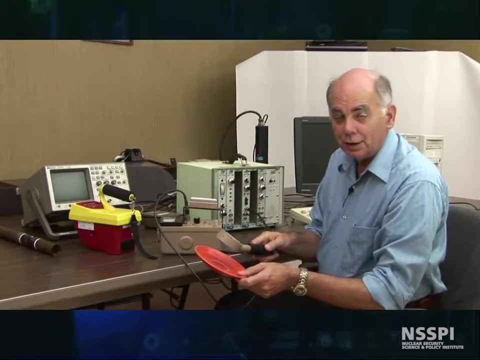 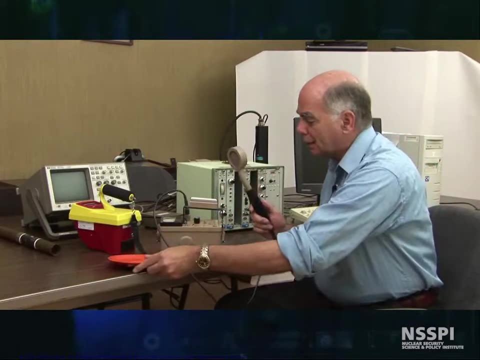 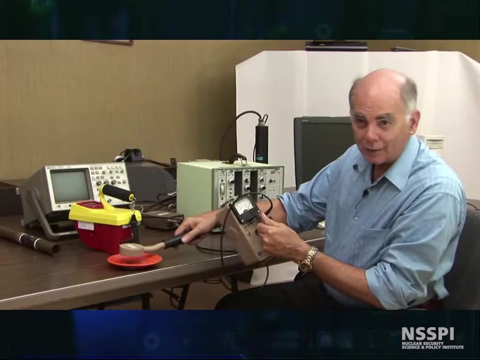 brought a source for us. This is Fiestaware and the nice orange color that you see there actually comes from uranium And to give you an idea of how radioactive it is on a times one scale, I can make this go off scale. 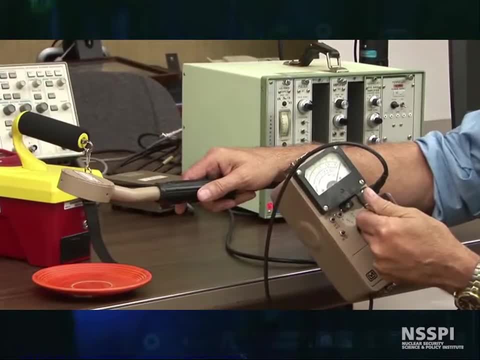 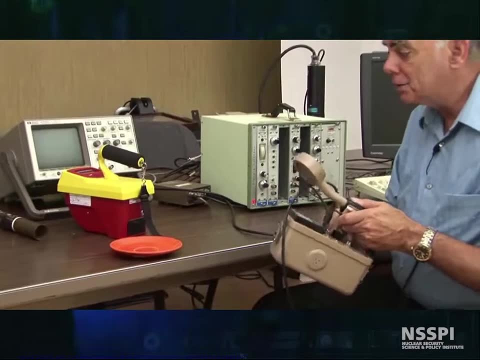 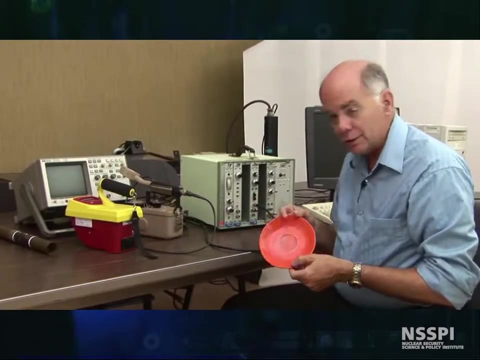 Okay, Well, that sounds pretty scary, and actually I must be a brave man to sit here next to this radioactive plate. but just between you and me, your grandmother probably ate breakfast off plates like this, and they managed to live a long and useful life, most of them. 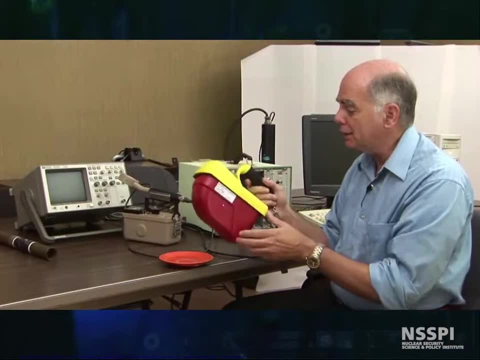 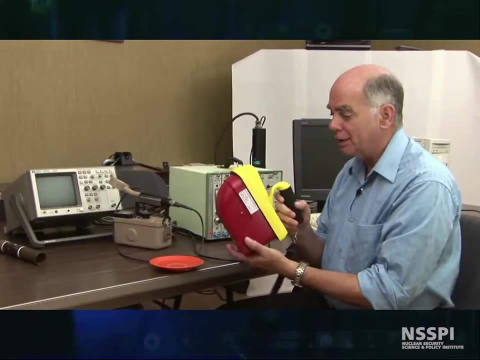 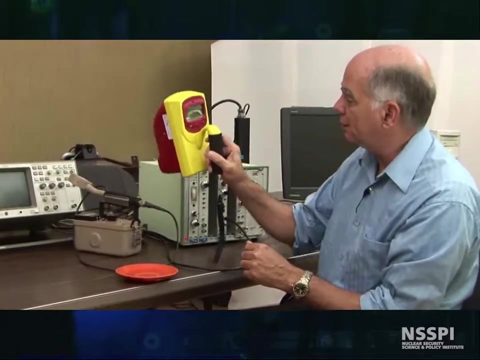 So if here's our second gas-filled instrument and this is an ion chamber, Inside here is a cylindrical chamber. It measures alpha, beta, gamma and has readings in micro R. Right now the radiation field is about 1 micro R- 1 to 5 micro R per hour. 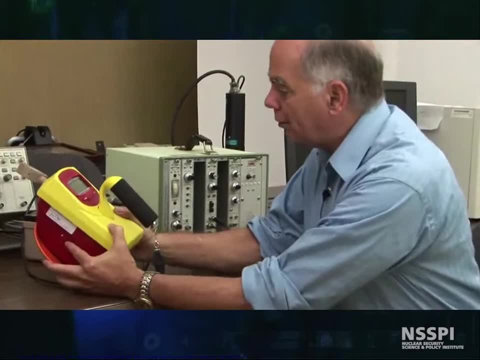 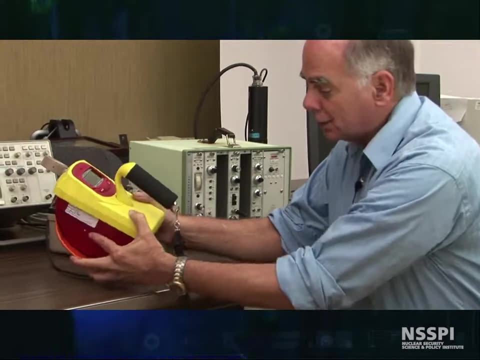 And if I set it on the plate, oh my gosh, we're up to 13,, 14,, 15 micro R per hour. So this gives you an idea of how simple it is to get an ion chamber to work on the surface. 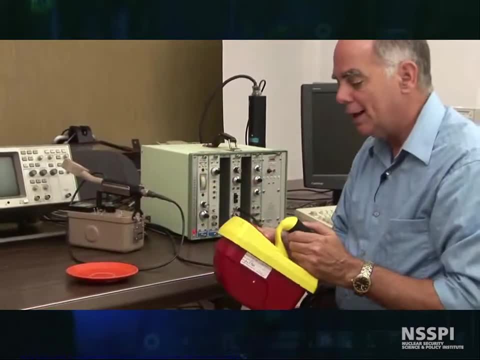 The first thing we need to do is put some water in the container. So here's our eye of the ion chamber And what I'm gonna do is I'm gonna put it over here. I'm going to sensitive the Geiger counter. is That what is a small, small fraction of your annual? 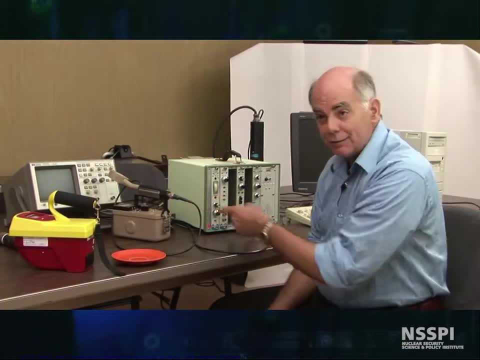 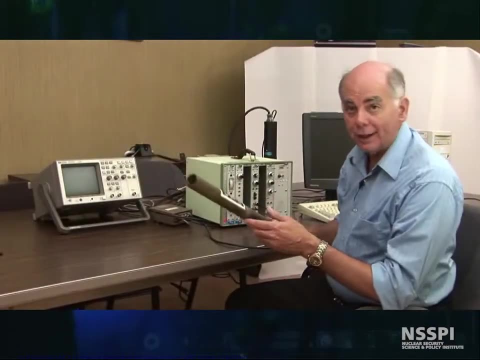 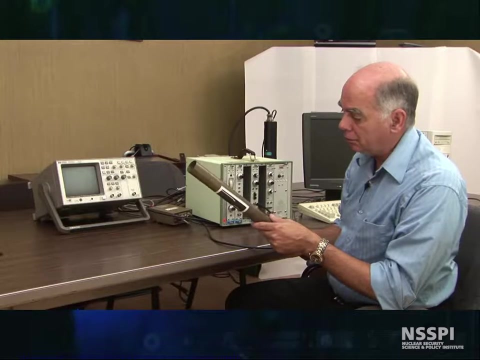 dose that you get from background radiation drives Geiger counters completely off scale. The next thing we're going, the next gas filled detector we're going to talk about are BF3 s, and this unassuming tube right here is a boron trifluoride neutron detector. as we talked,